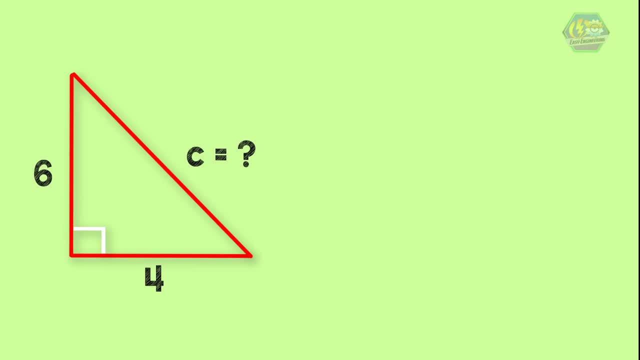 As we can see, the side c is the hypotenuse. therefore we can use the Pythagorean Theorem, which is: hypotenuse squared equal to the sum of the squares of two sides. So the equation will become: c squared equal to 6 squared plus 4 squared. 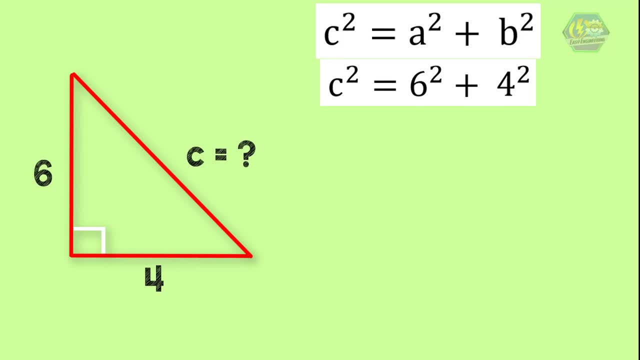 6 squared means 6 will be multiplied 2 times, and 4 squared also means 4 will be multiplied 2 times. Therefore, the equation will become c squared equal to 36 plus 16.. So c squared is equal to 52.. 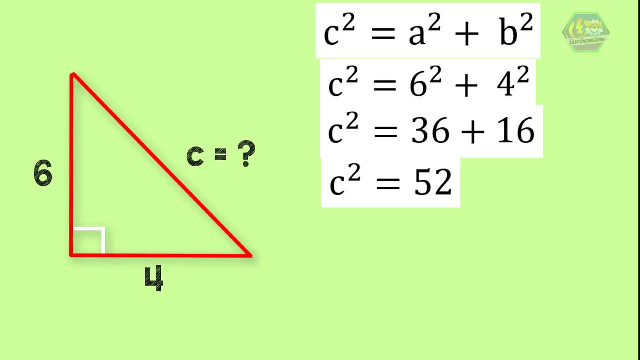 In order to find the c, we need to take the square root of both. Therefore, the square root of 52 is 2 square root of 13.. So the hypotenuse is equal to 2 square root of 13, or approximately 7.2.. 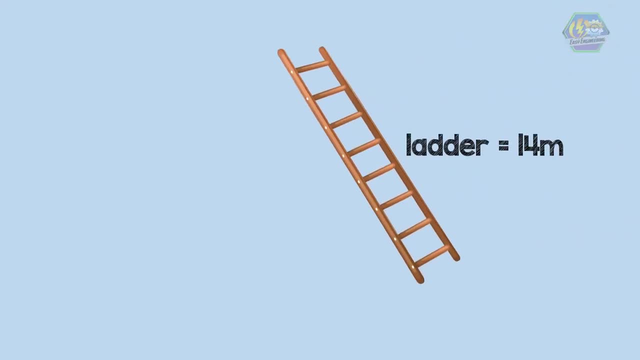 Now for another example. A ladder of 14 meters long is placed on the ground in such a way that it touches the top of a vertical wall of 36.. Therefore, we can easily find the distance of the foot of the ladder from the bottom of the wall. 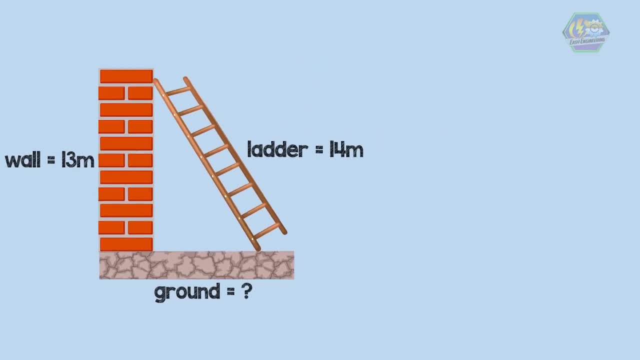 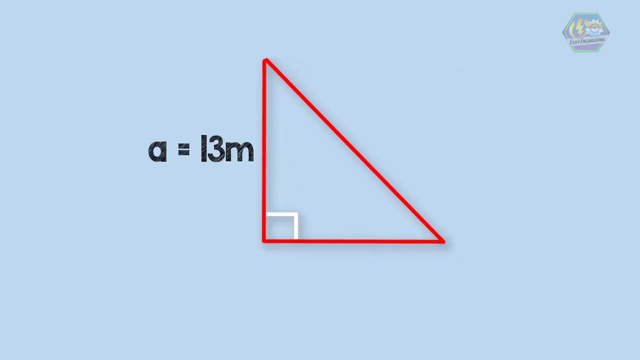 Take a look at the picture. You can see that the ladder which is placed on the ground and touches the wall forms a right triangle. Therefore, we can easily find the distance of the foot of the ladder to the bottom wall. Now let a equal 13 meters, which is the hypotenuse, equal to 14 meters, and b is the other side of the wall. 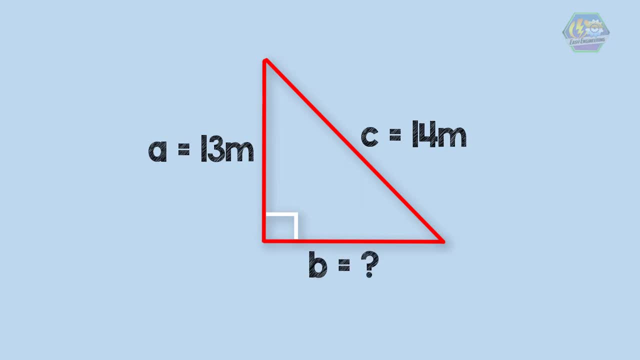 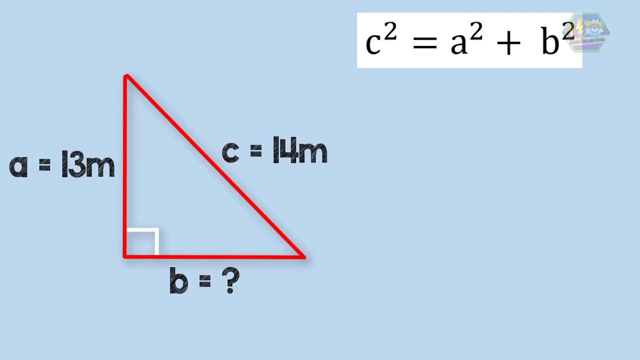 The other side of the triangle, which is the unknown. So, according to Pythagorean theorem, c squared is equal to a squared plus b squared. Therefore, by plugging in the values, the equation will become 14 squared equal to 13 squared plus b. 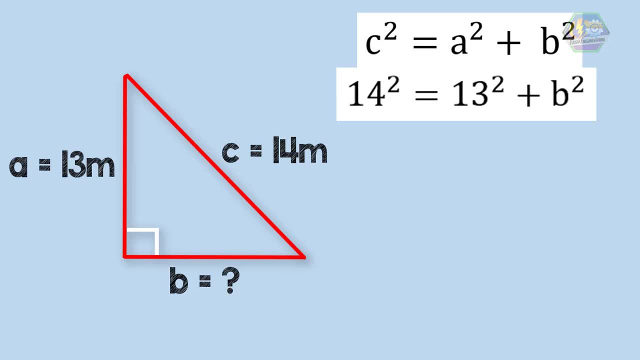 squared. Since we need to find the value in variable b, we need to transpose the equation. Therefore, the equation will become 14 squared minus 13 squared, equal to b squared. So b squared is equal to 27.. To find b, we need to take the square root of both sides. 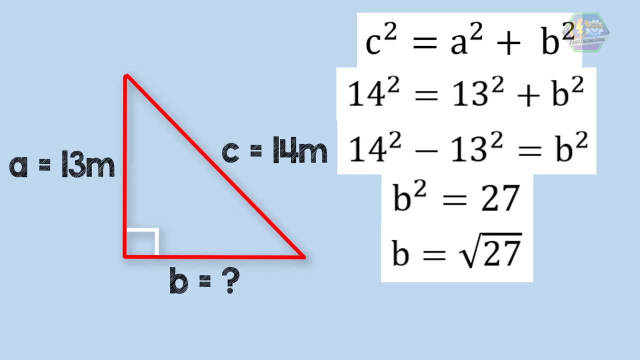 So it will become b is equal to the square root of 27.. Therefore, the distance of the foot in the ladder to the bottom of the wall is approximately 5.2 meters. So now that you finally know Pythagorean theorem, I encourage. 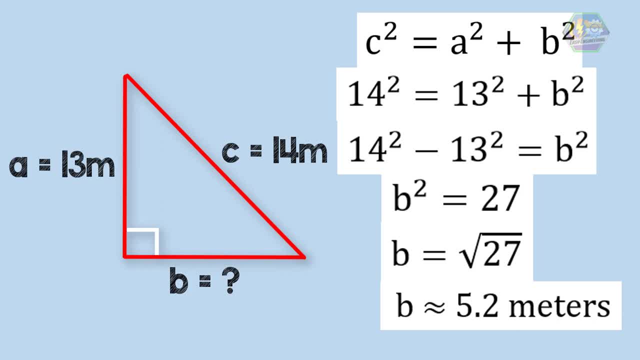 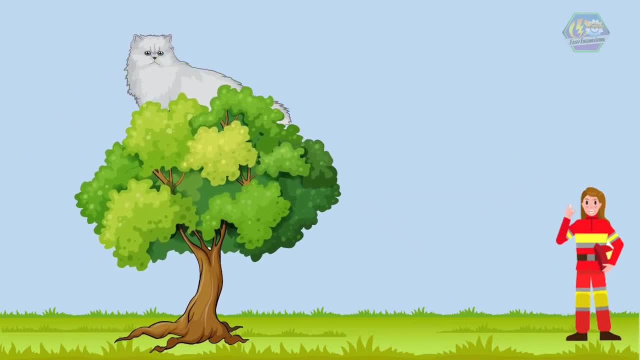 you to pause this video first and try to solve this problem. Jane is a firefighter saving a cat that is trapped at the top of the tree. She leans a 10 meters ladder against the tree. The base of the ladder is 3 meters from the top of the tree. 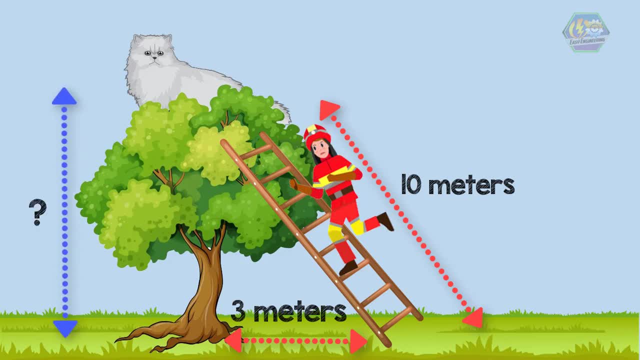 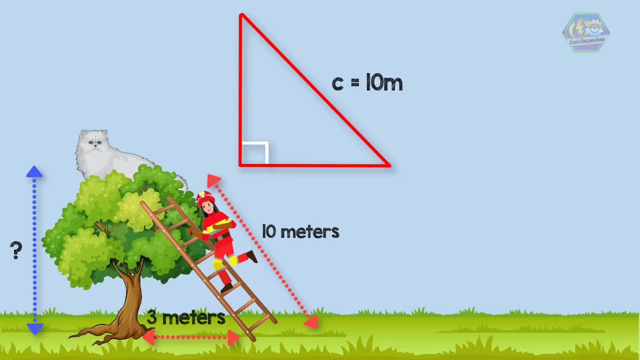 Now, how high is the cat? So we can use the Pythagorean theorem in solving this problem. The hypotenuse in the problem is the height of the ladder Which is leaning in the tree, and the other side of the triangle is the distance of the ladder to the tree. 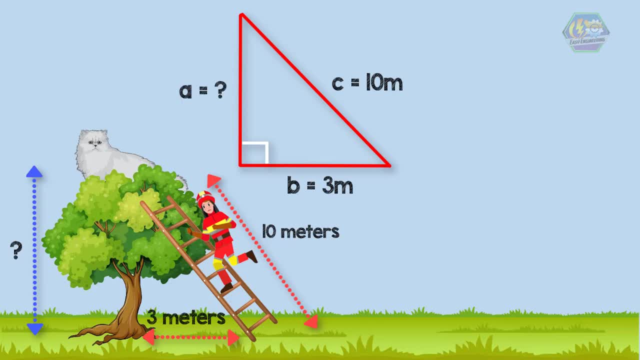 Now we are asked to find how high the cat is. Therefore, using the equation, C squared equals to A squared plus B squared, We can now find how high the cat is. So the equation will look like this: Therefore, the cat is at 9.54 meters high. 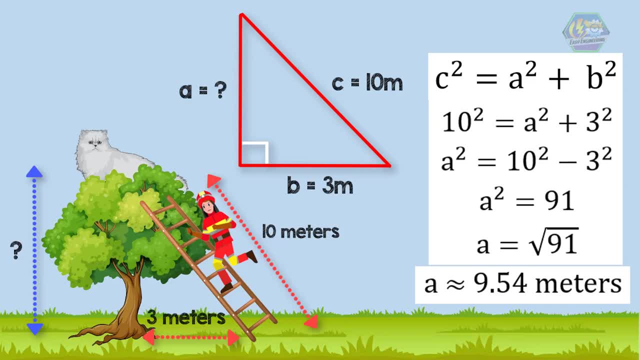 Do we have the same answer. So what can you say about the Pythagorean theorem? Easy right, That's it, guys. I hope you learned a lot about Pythagorean theorem. You can also watch our other videos here. Once again, this is Easy Engineering. We make engineering topics easy and fun for you. 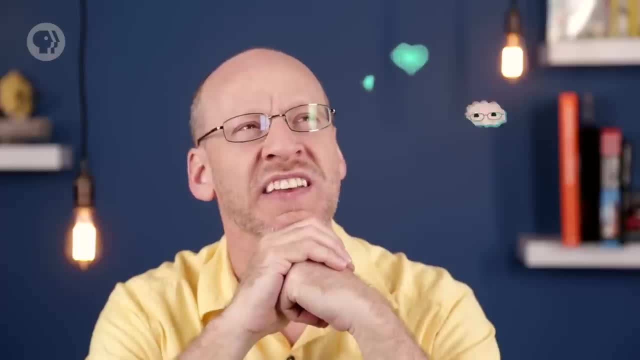 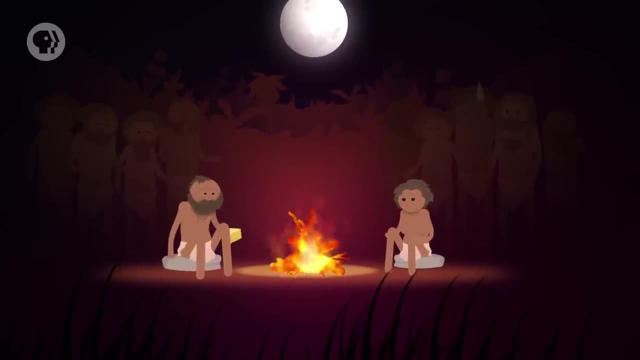 What is the nature of the universe? How's that for a question? For a long time, we humans had no idea what was going on in the universe. To help, we made up stories to either help us explain what we saw or to make us feel better about what we didn't understand. But then science came along and